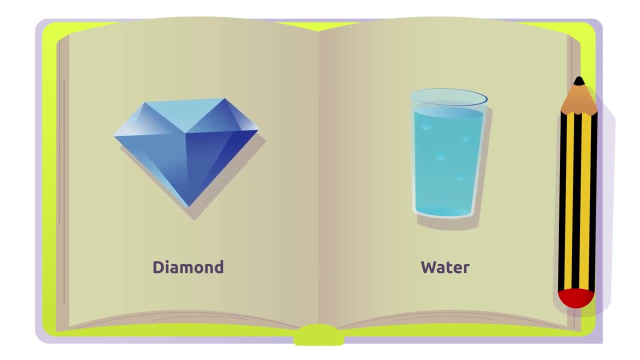 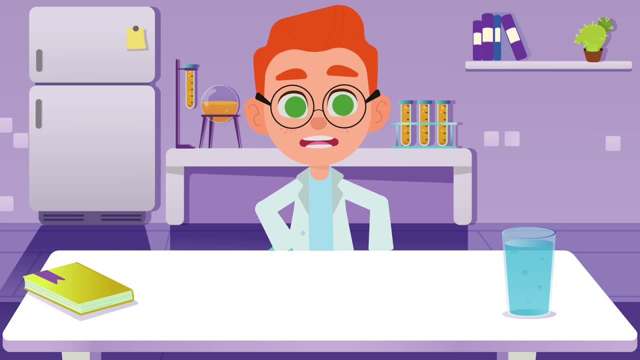 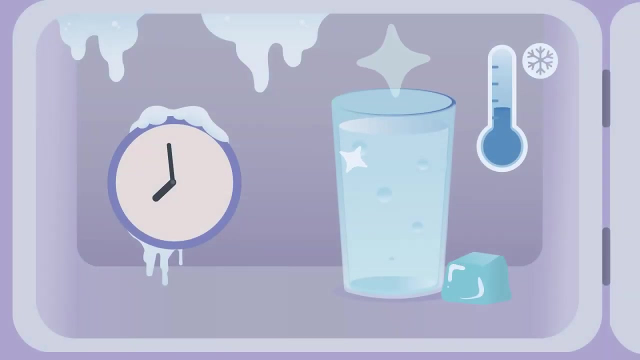 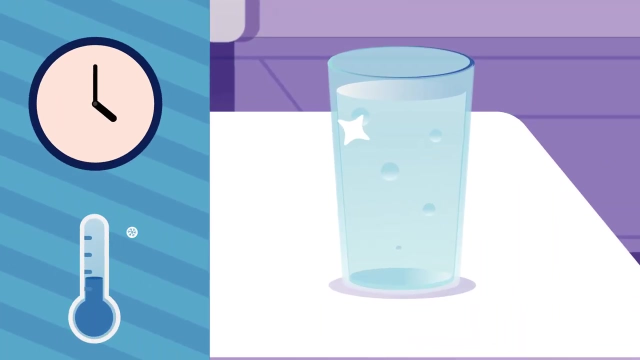 In a physical change, the composition changes. The composition of these substances wouldn't be altered. Look at this glass of water. If I place it in the freezer, the water will turn into ice because of the very low temperature. But if I took the glass of water out of the freezer, the ice would melt, turning into water again. 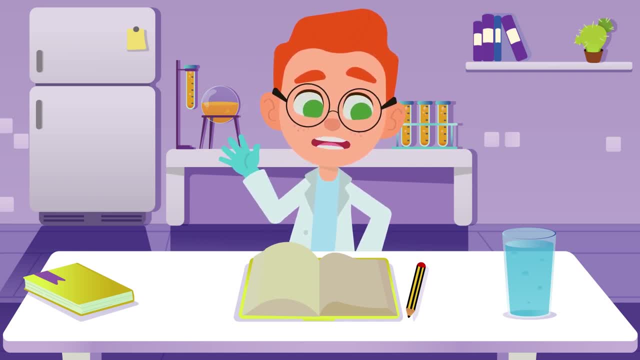 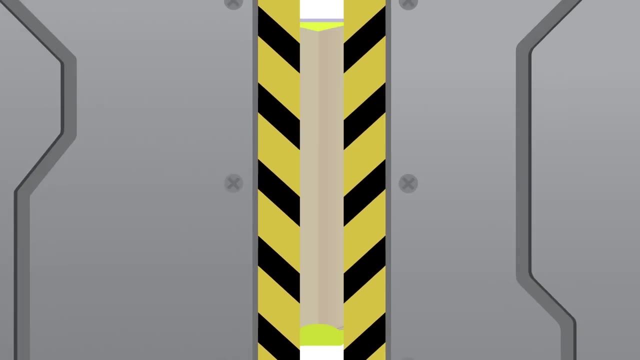 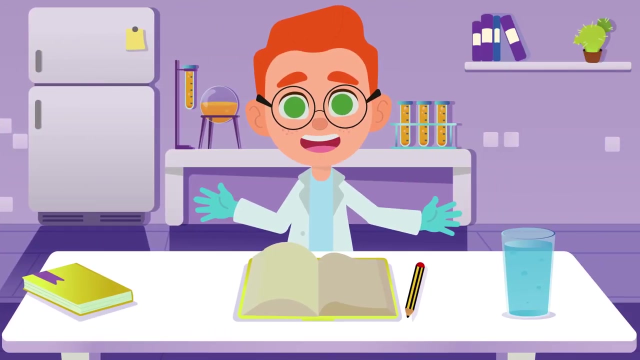 This is a physical change, but the substances change. This is still the same Interesting. right Now let's take a closer look at mixtures. Mixtures- A mixture, is a combination of two or more pure substances. There are two types of mixtures: homogeneous and heterogeneous. 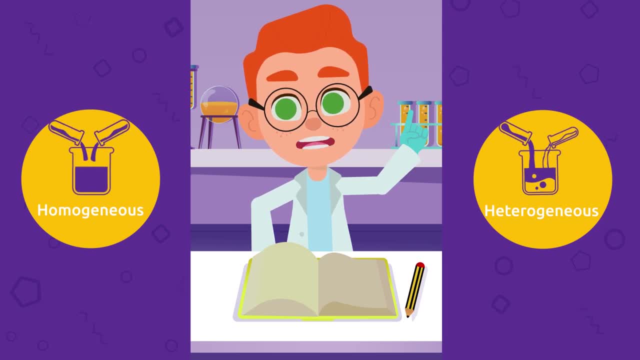 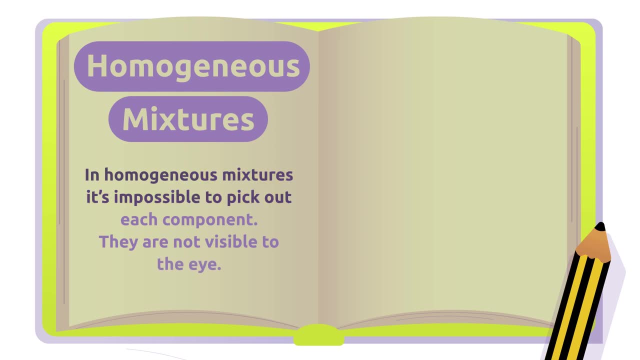 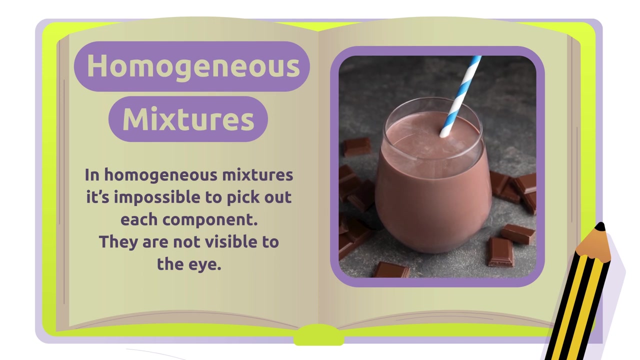 Let's look closer at each one of these two groups. In homogeneous mixtures, it's impossible to pick out each component. They are not visible to the eye. Solutions like water with salt or chocolate milk are homogeneous mixtures. Can you think of another example of a food that is a homogeneous mixture and that we use a lot in cooking? 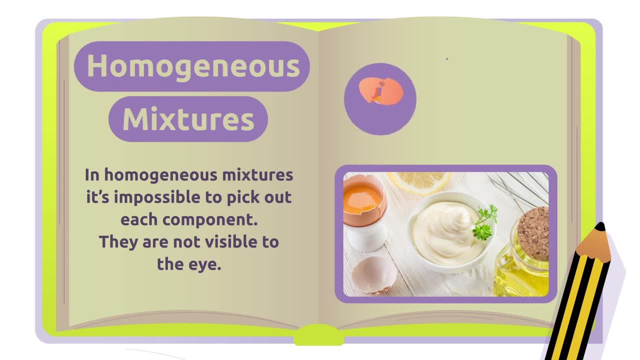 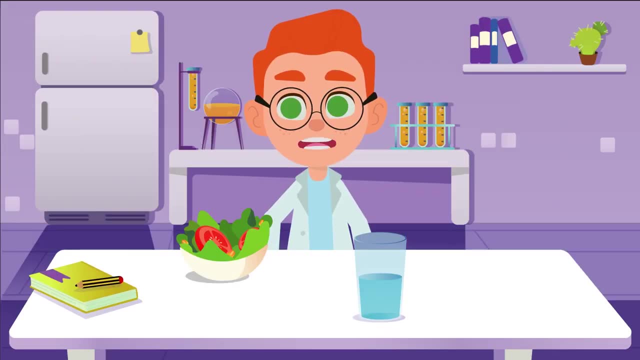 Mayonnaise is a great example. It's made with eggs, oil and salt. In this case, substances can be found in any state of matter: solid, liquid or gas. An example of this would be water with oil or salad. 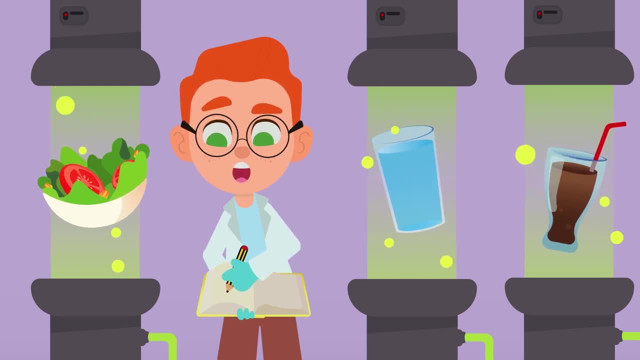 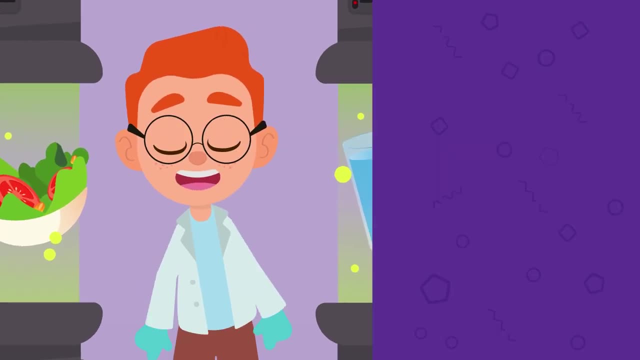 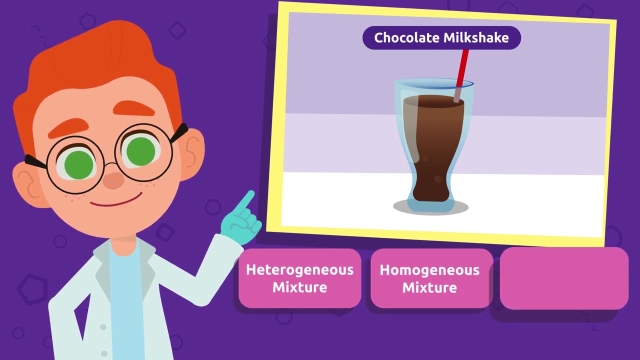 I'm trying to write all this down. I don't want to miss anything. Would you like to practice what we learned? Come on, let's classify these substances and mixtures together. What do we have here? Wow, Chocolate milkshake. 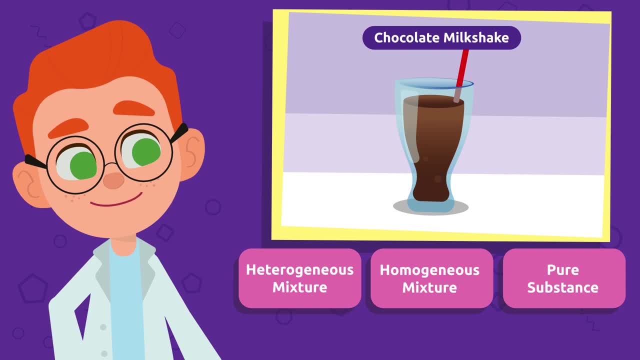 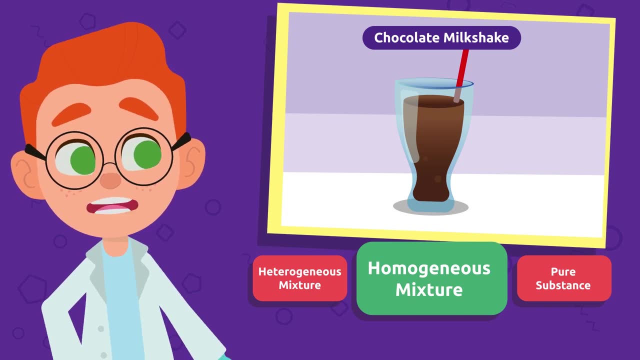 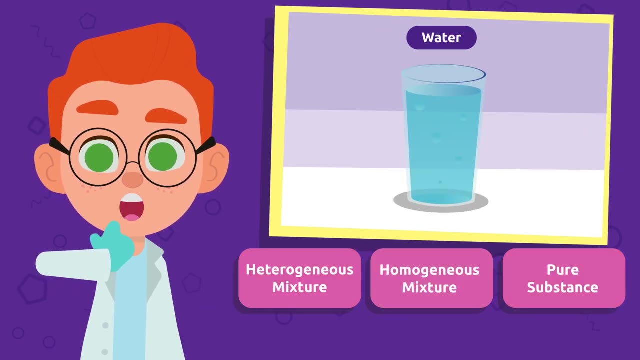 What kind of substance or mixture is it? This chocolate milkshake is a homogeneous mixture because its components can't be seen with the naked eye. It's water. Hmm, didn't you remember what type it was? This is a very simple type of substance.